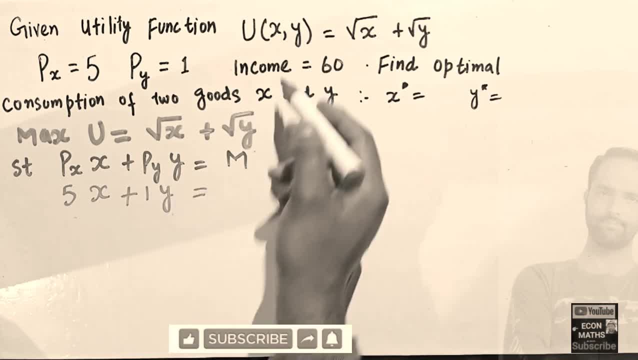 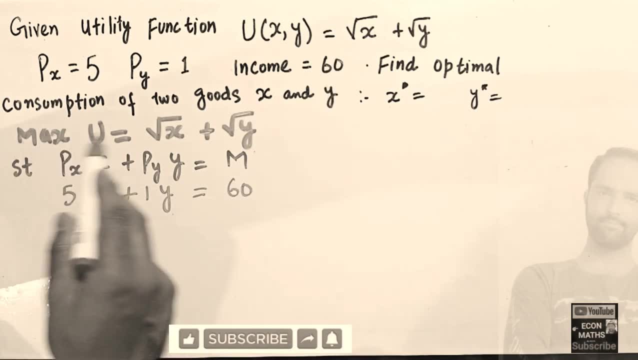 Times y should be equal to the total income of the consumer, which is 60 here. So in place of m we have 60. So we want to maximize this utility function subject to this budget constraint. Now, first order condition. for you know, optimization requires that our marginal rate of substitution between two goods, x and y, should be equal to their prices. 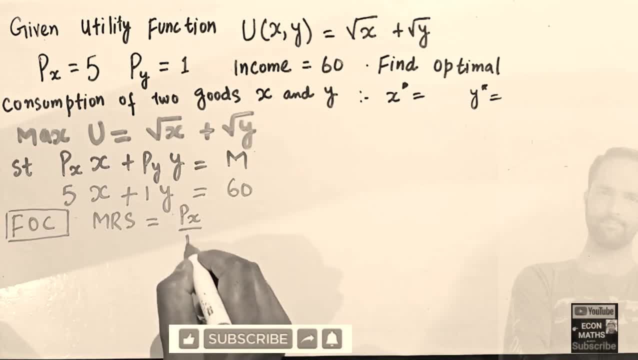 Ratio of their prices. That means price of x upon price of y By MRS. what we mean, MRS, means to find the marginal utility of good x upon marginal utility of good y. Okay, So we need to find out. Marginal rate of substitution is simply the marginal utility of x upon marginal utility of y. Okay, 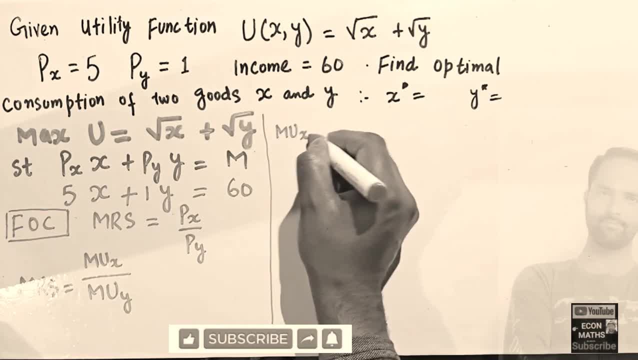 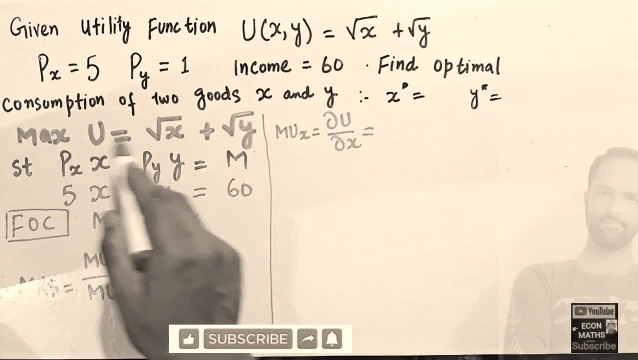 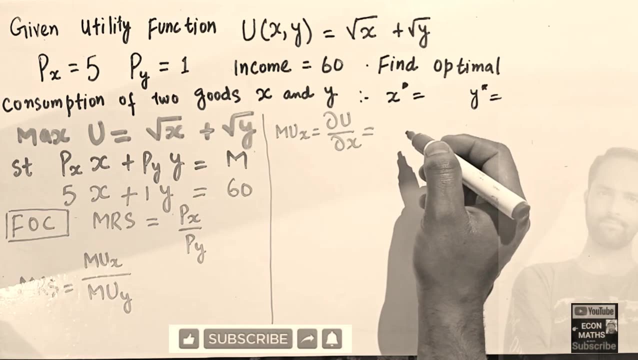 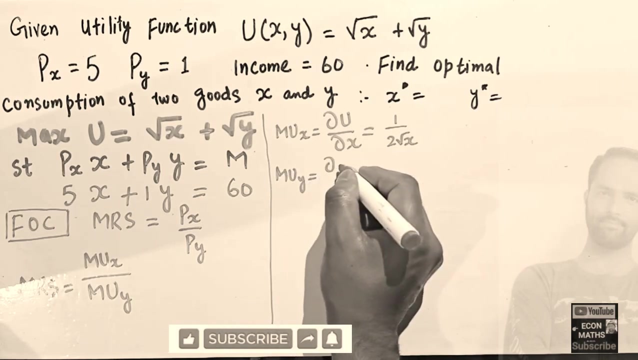 And what will be the marginal utility, Marginal utility of x? simply the partial derivative of utility function with respect to x. So this is our utility function. Let's take its derivative with respect to x. So derivative of under root x comes out to be 1 upon 2 under root x. This is the derivative of this under root x. Similarly, marginal utility of good y will be the partial derivative of good y. Okay, 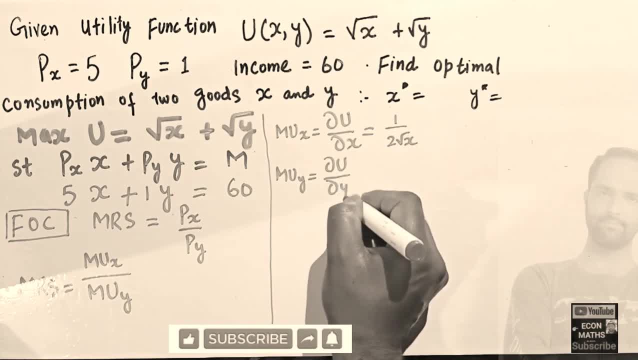 Smackn Rs is equal to tactical Cross тоже. there You should be within the area of the particular unit student. the particular unit student of the particular unit. student at the ballpark. let's suppose that an integral of utility function with respect to y. So we are taking the derivatives with respect to y here. So the derivative of this term is 0. derivative of under root 5 will be 1 upon 2 under root. 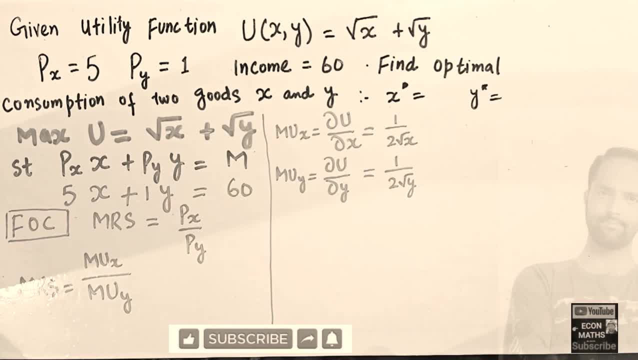 And we take the derivative of y instead of y. Right, remember, theited negative derivative of inter Lor beach can go along with the derivative of y under root and you should get the derivative of this element in general, as if we are taking from the derivative of y or by NF of, and we get this so. 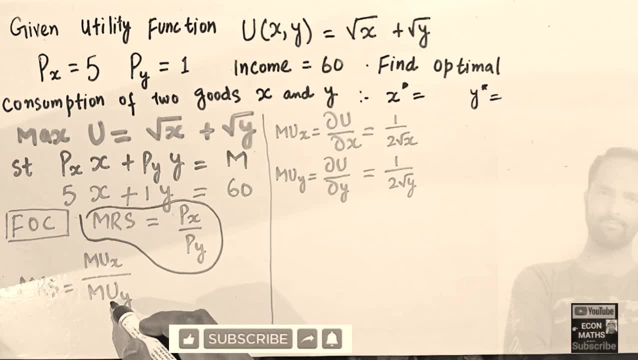 st is beneath root es so less inter l large left than 3.. Or the derivative of is 0 and재 root of y will be one upon Known under roots Known, the dilution of y- K. So our equilibrium condition is this: 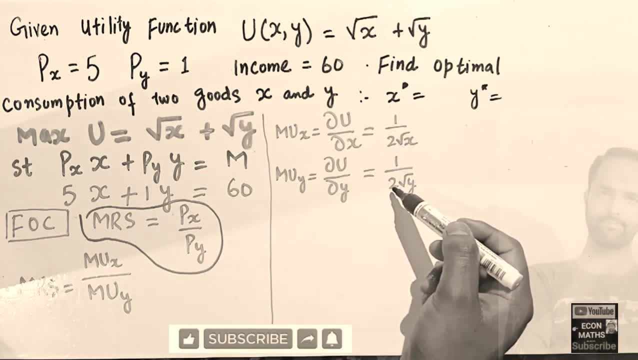 OK, may use this condition To ride marginal utility of x. this is marginal utility of y. that means using this condition here. that means in place of m u x, i will write 1 upon 2. under root y divided by marginal utility of y is: 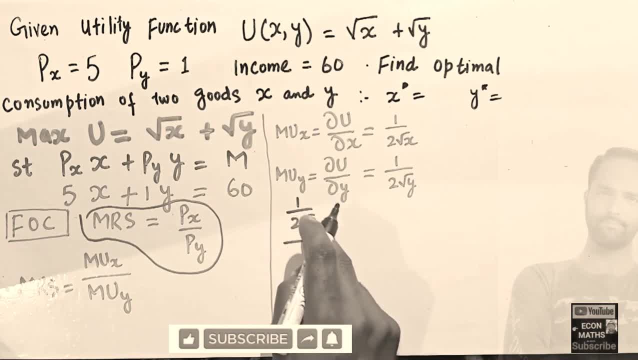 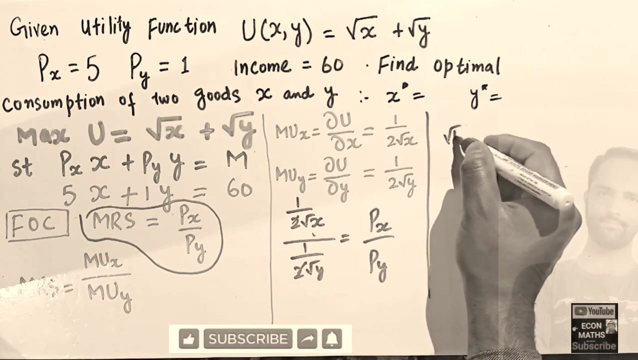 equal to- sorry, we have here x. okay, marginal utility of x. so here we have 2. under root y should be equal to the ratio of the prices p of x upon p of y. so when we solve this, 2 and 2 will get cancelled. we are left with under root y. 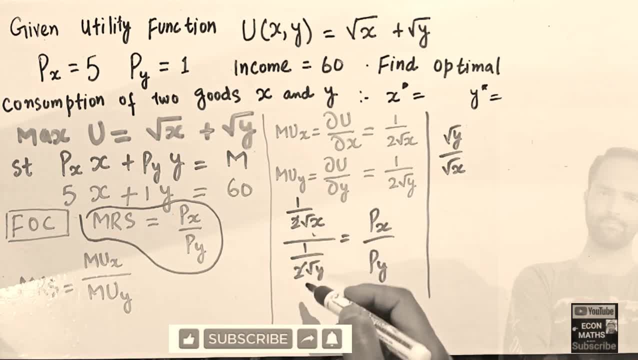 upon under root x. okay, when we transpose this to the numerator it will get reciprocated, so we will get: y upon x should be equal to p of px upon py. so price of good is 5, good x is 5, price of good y is 1. so we are left with 5 upon 1. so we can write it like this: 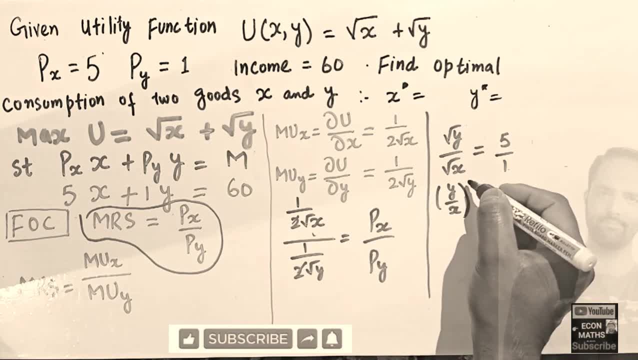 y upon x under root. so in place of under root we can write one half also. okay, should be equal to this, which gives us: y upon x will be transposing exponent. it will get reciprocated, so it will become 5 square here. that means y upon x is equal to 25. 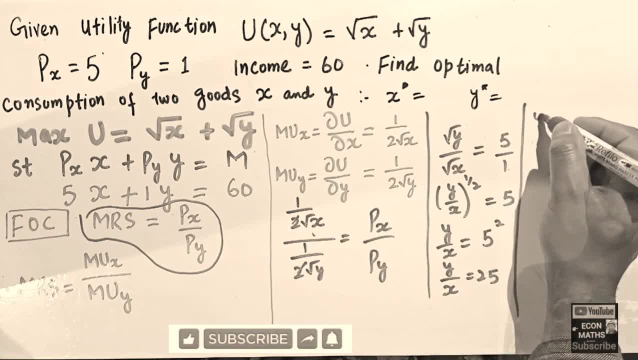 use us, y is equal to 25 times X. okay, that means Y is equal to 2: 25 times X. just plug this value into the budget constraint so we have for you X plus 1 times Y. value of Y is equal to 25 x. so again, 25 x should be equal to 60. so 5 x plus 25 x comes out to be 30. x is equal to. 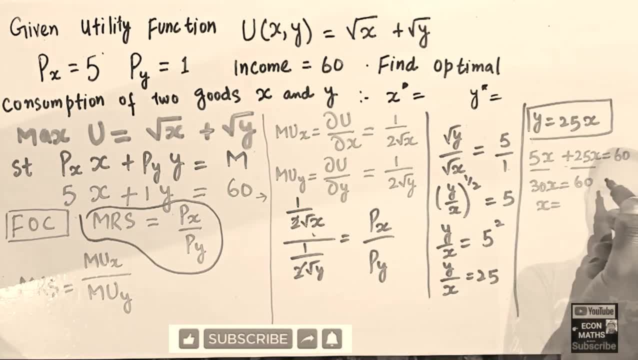 60, which gives us x is equal to, so 31s are, 32s are, so consumer will consume two units of good x. and what about the you know, units of good y? plug again: the value of x is equal to 2 in this equation. so we have 5 into 2, plus y should be equal to 60. so 5, twos are 10, we are left with y.